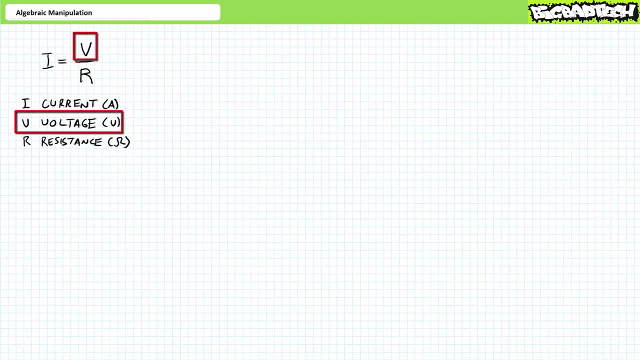 is equal to voltage, symbolically represented as a V measured in the units of volts divided by. resistance, symbolically represented as R, measured in units of ohms- Kind of this funny shaped horseshoe thing- If you've got known voltage and known resistance. 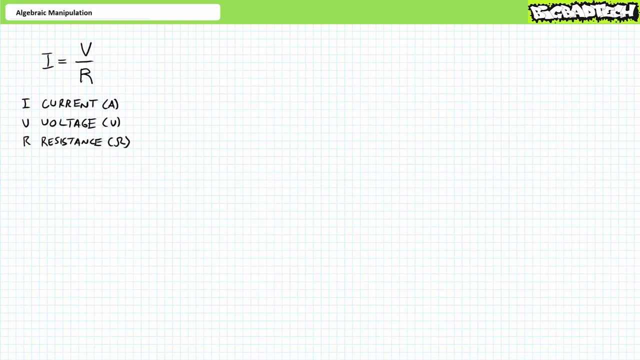 one simply divides voltage by resistance and obtains current units of amps. For example, given a known voltage of, let's say, 14.3 volts across a 240 ohm resistor, an application of Ohm's law demonstrates one might expect roughly 59.6 milliampers of current. 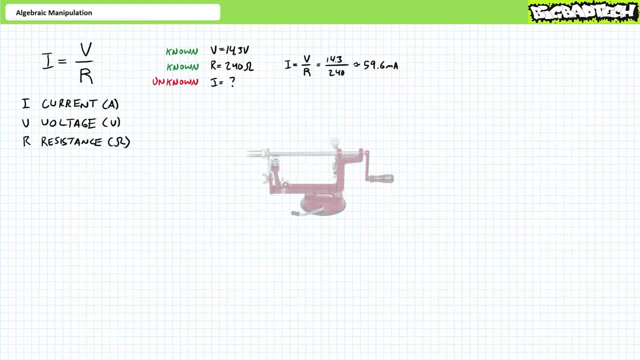 to travel through it Too easy. An equation like this is a machine as complicated as an apple peeler. It has inputs- voltage and resistance. It performs some operation. voltage divided by resistance: It has an output current. We explored this level of calculation. 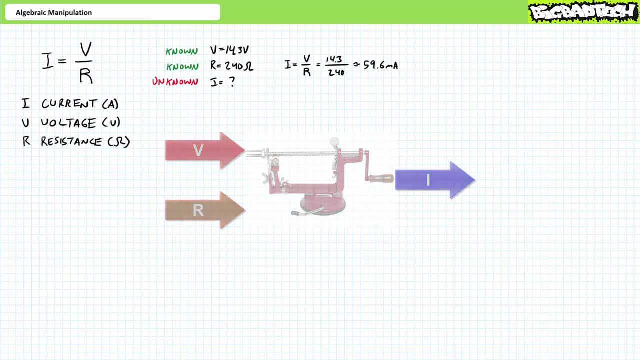 in the aforementioned DC math lecture, and this should be well within your ability level. Not all the time we were presented with such a perfect setup. Sometimes we know voltage and current but not resistance. or maybe we know current and resistance but not voltage. 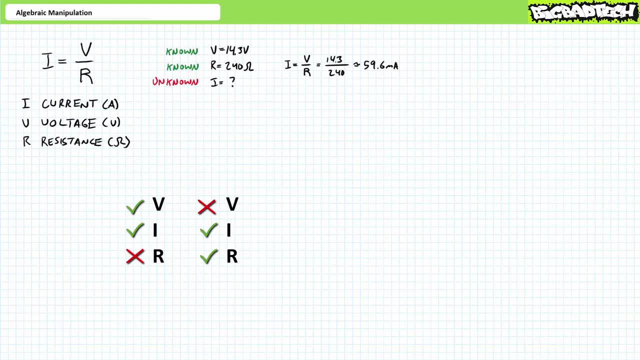 No problem, One can always algebraically manipulate a given equation to solve for unknown properties given known inputs. Allow me to demonstrate using Ohm's law. Let's say we know current I and resistance R and want to use these properties to solve for voltage V. 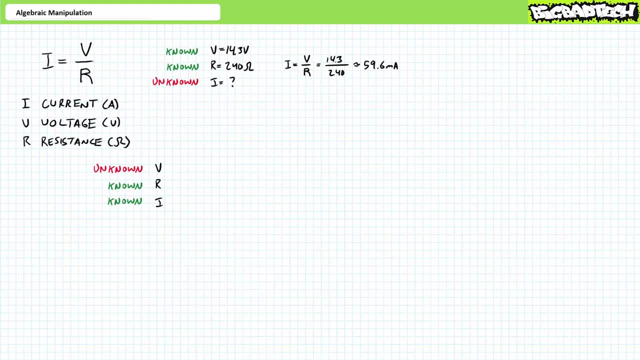 The goal of algebraic manipulation is to isolate all the knowns on one side of an equation and all the the unknowns on the other. Given our present understanding of Ohm's law, known entities I and R need to be on one side of the equation. 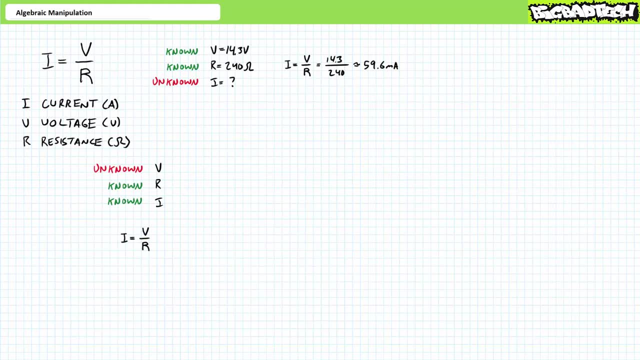 and unknown quantity V on the other. One doesn't just move these quantities around without restriction, but rather one follows rules regarding their movement, The single most important rule being the equal sign. One can arrange and rearrange any equation in any fashion you wish. 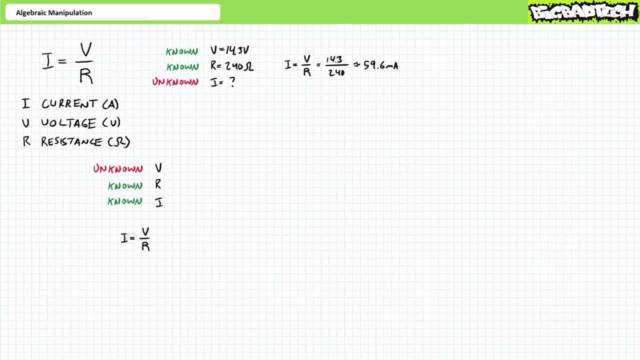 However, equality must be maintained at all times. That's the point of equality- Equations like Ohm's law. There exists a real, observable relationship between these properties and any upsetting of the quality means you're making things up. Equality must be maintained. 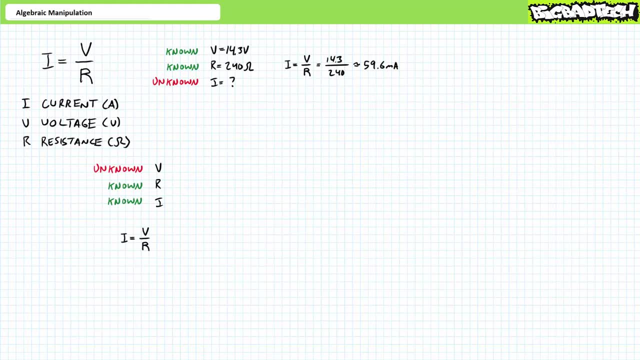 Here's the general rules to maintaining equality. They all share a common trait. See if you can identify the shared trait. One can add any quantity you wish to one side of the equation. However, you must also add the same quantity to the other side of the equation. 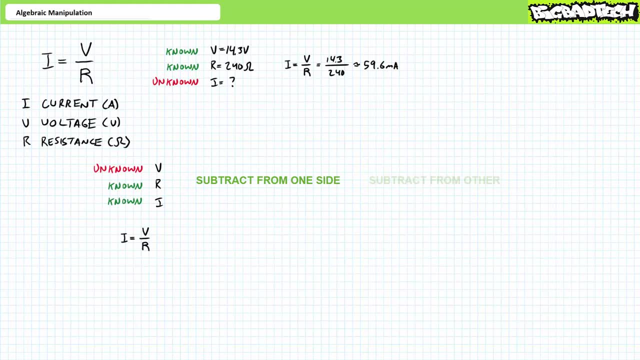 One can subtract any quantity you wish to one side of the equation. However, you must also subtract the same quantity to the other side of the equation. One can multiply one side of the equation by any quantity you wish. However, one must also multiply the other side of the equation. 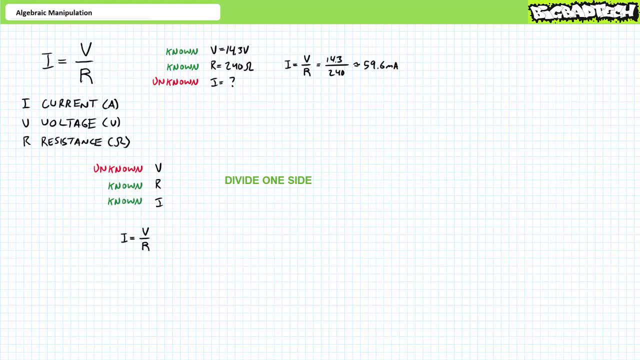 by the same quantity. One can divide one side of the equation by any quantity you wish. However, you must also divide the other side of the equation by the same quantity. One can raise one side of the equation by any power you wish. However, you must also raise the other side of the equation. 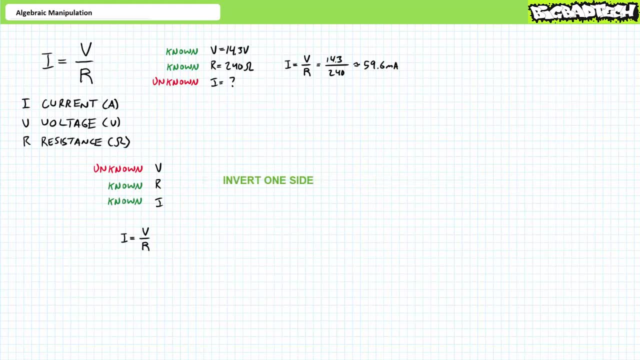 by the same power. One can invert one side of the equation. however, we must also invert the other side of the equation. Have you figured out the pattern yet? For those of you who haven't, here: it is To maintain equality. one must do to one side what is done to the other. 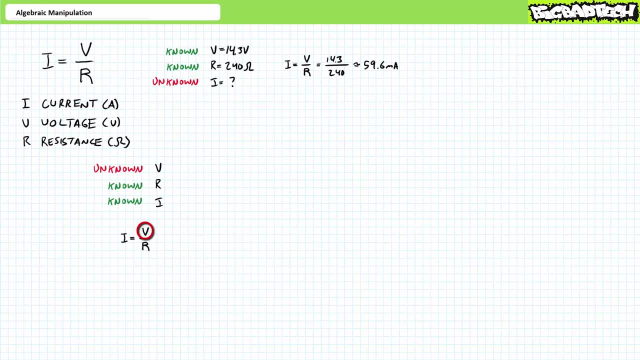 We need to isolate unknown property v on one side of the equation, As presently illustrated, it's being divided by r. What's the opposite of division: Multiplication. Multiply both sides by r. r cancels out on the right, And we're left with an equally valid permutation of Ohm's law which states: i times r equals v. 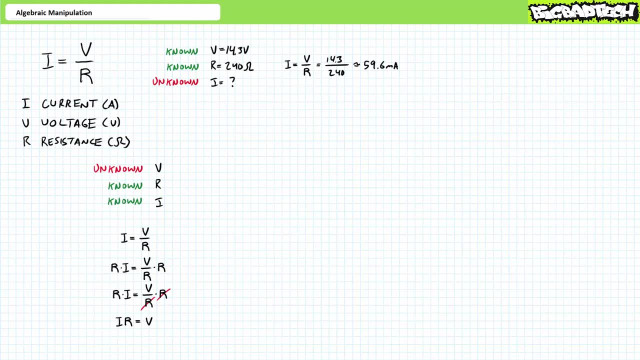 One can substitute in known values for i and r and determine unknown quantity v. Other equally valid permutations of Ohm's law exist. For example, let's say we knew v and i and wanted to solve for unknown quantity r. We've got a couple different starting points. 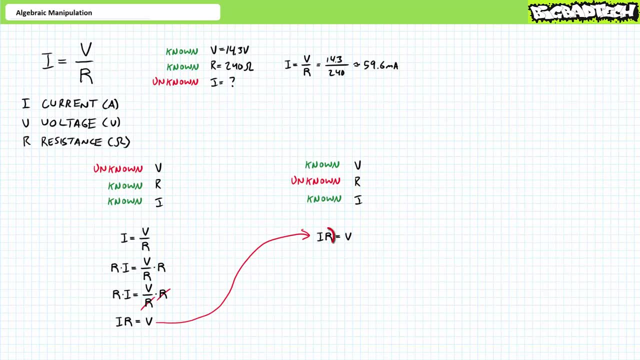 Let's begin with our second permutation, The first permutation of Ohm's law. As presently illustrated, we need to isolate the unknown property r on one side of the equation. r is presently being multiplied by i. What's the opposite of multiplication? 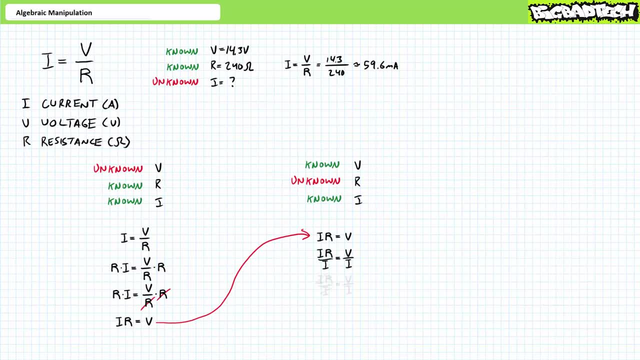 Division Divide both sides by i. i cancels out on the left, And we're left with yet another, equally valid permutation of Ohm's law, which states: r equals v over i. One can substitute in known values for v and i and determine unknown quantity r. 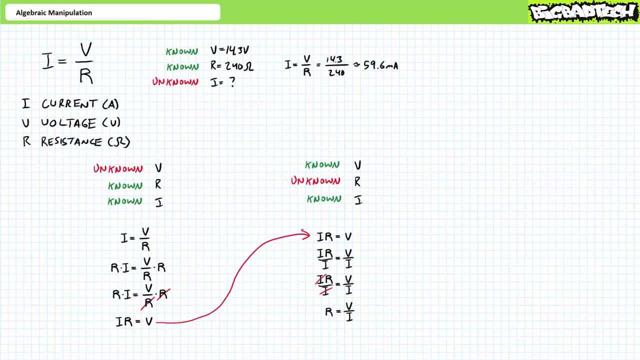 Note one needn't use the second permutation to arrive at the third, but rather proceed from first to third directly. Importantly, it should yield the same result. Allow me to demonstrate Using the original statement of Ohm's law. we again need to isolate the unknown property r on one side of the equation and known properties v and i on the other. 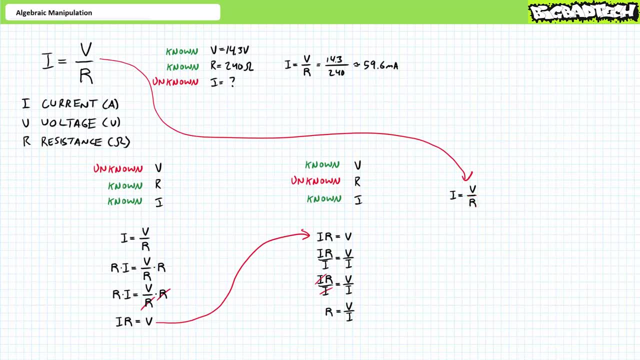 As presently illustrated, r is in the denominator. I do not like that. Let's invert both sides. Inversion means we flip both sides. We're left with 1 over i equals r over v. Unknown property. r is being divided by v. 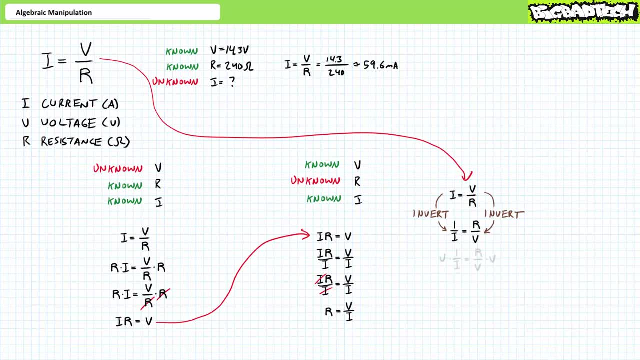 What's the opposite of division: Multiplication. Multiply both sides by v. v cancels out on the right And we're left with the identical permutation of Ohm's law which states r equals v over i. One can substitute in known values for v and i and determine unknown property r. 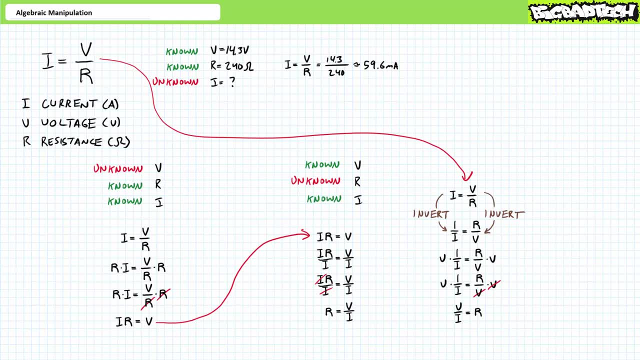 Note, in all of these manipulations, I'm giving myself an indication of those steps I've performed in the past. I might seem unnecessary given this simple expression, but trust me in a more complicated expression. this is a great way of leaving yourself a trail to backtrack if you mess it up. 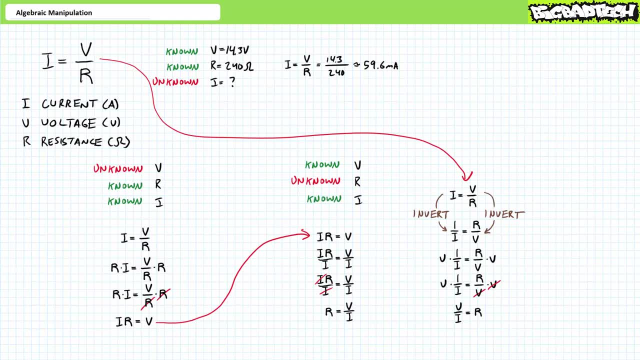 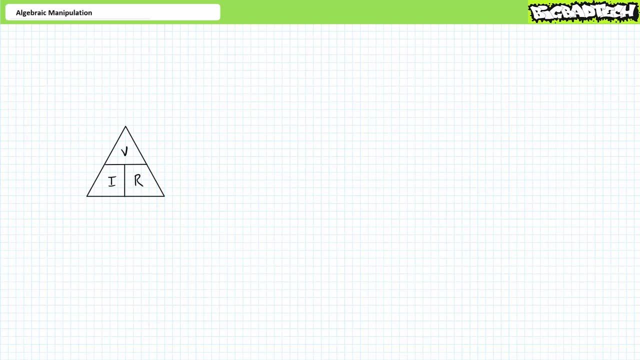 While we're still looking at this simple three-variable expression, let me show you a great shortcut for algebraic manipulations of similar types of expressions. Consider the three properties central to Ohm's law v, i and r, illustrated inside a triangle. 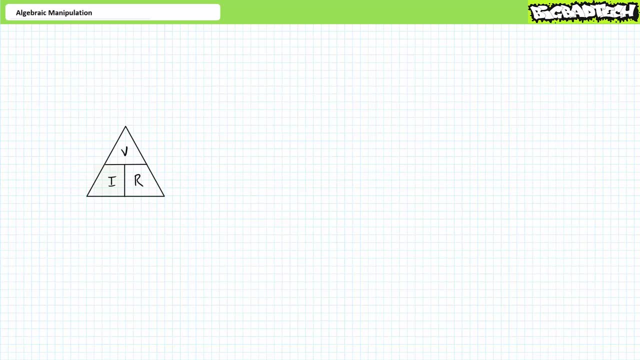 Let's say i is our property of interest Covered up, i is equal to v divided by r, because v is over r. This is our original statement of Ohm's law. What if v was our property of interest Covered up? v is equal to i times r, because i is next to r. 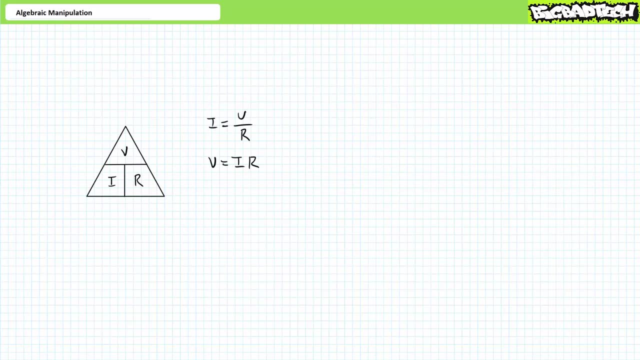 This is the second permutation of Ohm's law. Similarly, what if r was our property of interest Covered up? r is equal to v divided by i, because v is over i. This was our third permutation of Ohm's law. For simple three-variable expressions, let's look at the following. 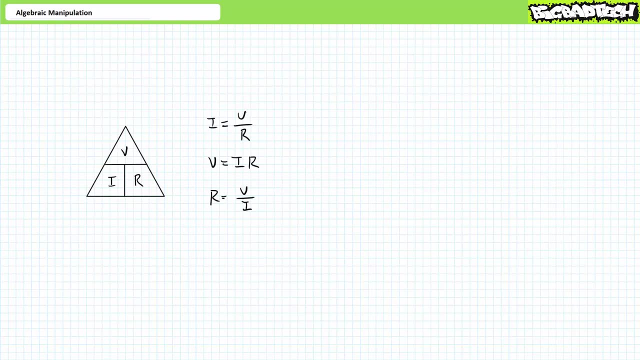 The first permutation is for Ohm's law, The second is for Naive's law, The third is for Yang's law, The fourth is for Laplace's law. If we consider the third one as our property, we're going to be able to know the answer with thisitive equation: 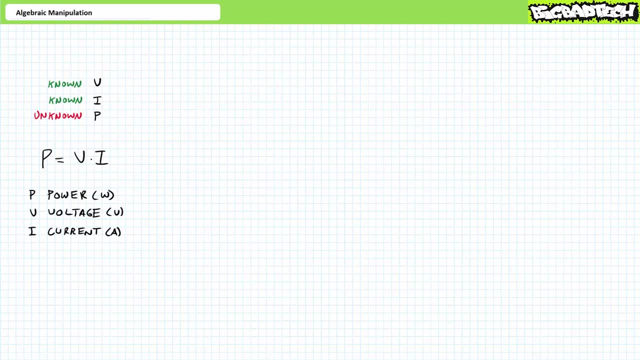 The first term of the third erklären that the two equations of Ohm's law are similar. In the view of the second term, we compute the current of two equations of ohms and in the view of the third term, we equal the current of uh and u, which gives us the expression of the order of the two equations of ohm's law. 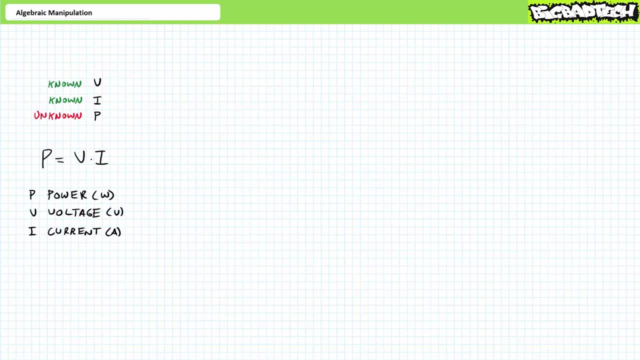 This is a lightning fast means of algebraically manipulating equations to solve for the desired unknown property. Put your understanding of this concept to the test with this series of illustrated examples of the dc power equation, something we'll examine in greater detail in the near future. 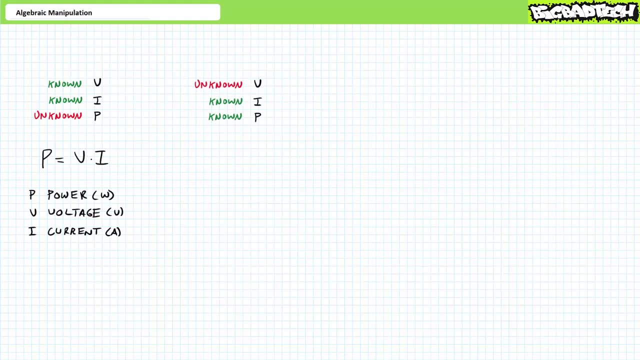 See if you can algebraically manipulate this equation to solve for v, given known inputs p and i. Similarly see if you can algebraically manipulate this same equation to solve for unknown quantity, i, given known p and v values. By all means, pause the lecture and try this on your own. 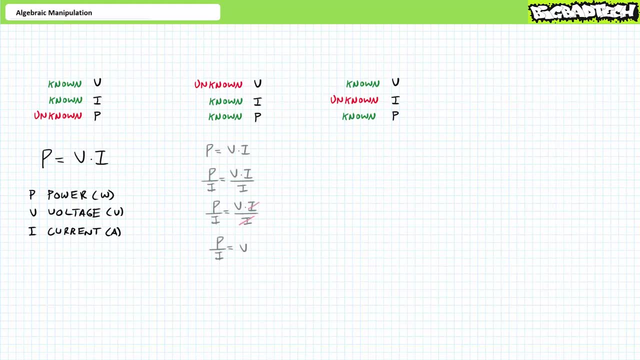 If you're tracking, you should have obtained the following results: Given p equals v times i. an algebraic manipulation of this equation demonstrates that v is equal to p over i. Given known p and i values, one can solve for unknown v by dividing p by i. 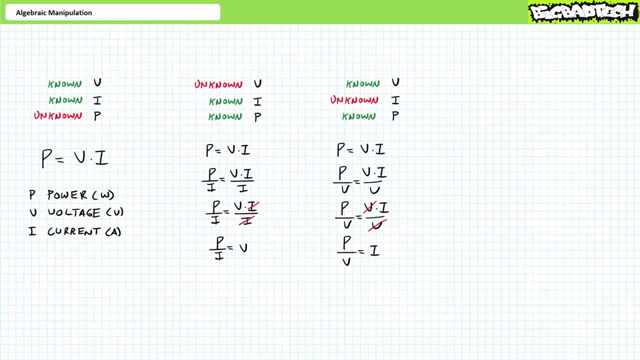 Similarly, an algebraic manipulation of the original or the second permutation demonstrates that i is equal to p over v. Given known p and v values, one can solve for unknown i by dividing p by v. That wasn't too hard, was it? 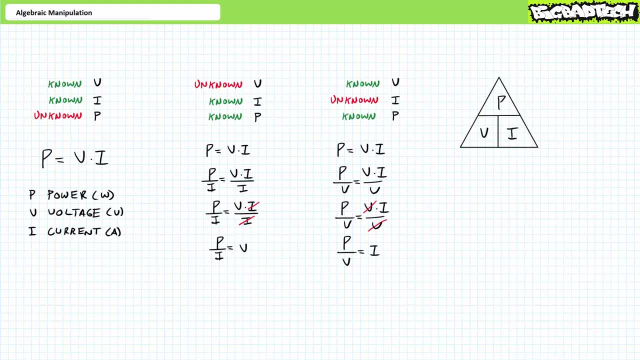 Again, the triangle method works equally well here. Overlay p, v and i in a triangle. Let's say p is our property of interest. Cover it up Okay. P is equal to v times i, because v is next to i. 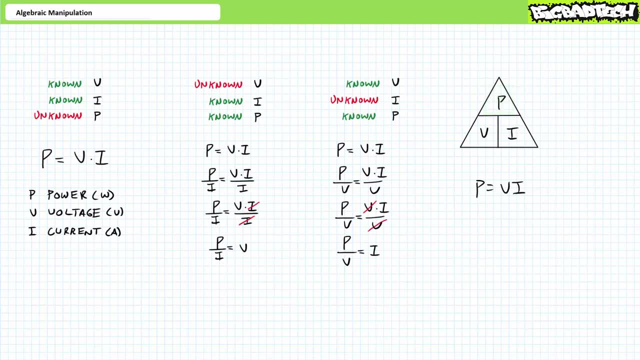 This was our original permutation of the DC power equation. What if v was our property of interest? Cover it up. V is equal to p divided by i, because p is over i. Similarly, what if i was our property of interest? Cover it up. 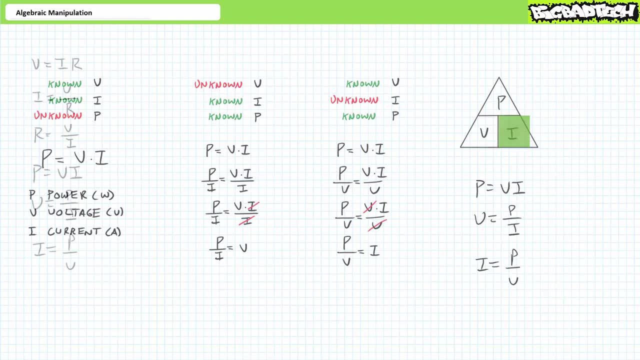 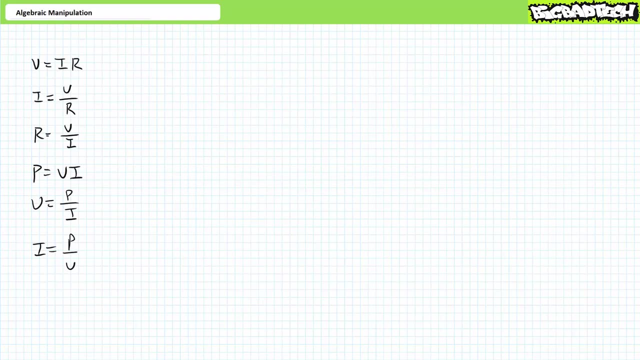 i is equal to p divided by v, because p is over v. All right, let's turn up the heat. Not all the time we are presented with such simple expressions, and sometimes we need to synthesize two expressions into one. The case in point: Ohm's law and the DC power equations. 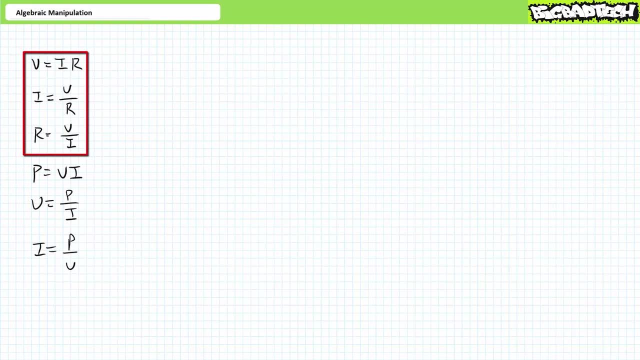 Thus far, we have three permutations of Ohm's law: v equals i times r, i equals v divided by r and r equals v divided by i. Additionally, we have three permutations of the DC power equation: p equals v times i, v equals p divided by i and, finally, i equals p divided by v. 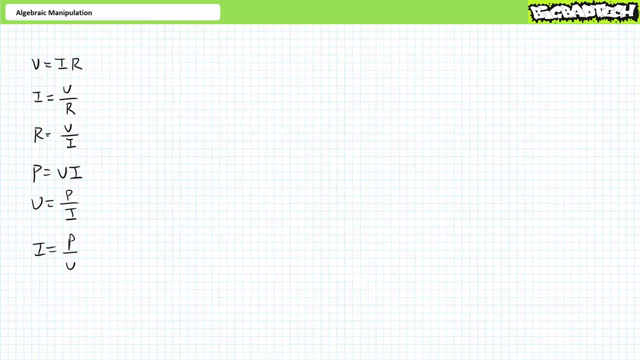 Given these six equations deal with the same properties, can we use them to divide other valid relationships between p, v, i and r? Let's do that, Okay. Indeed, we can. For example, given known v and known r, can we solve for unknown p? 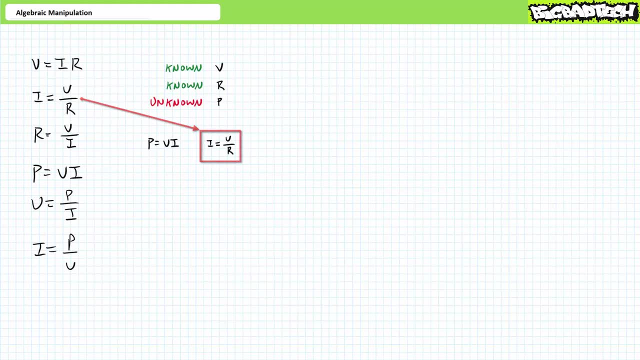 Consider one permutation of Ohm's law which states i equals v over r and a permutation of the DC power equation which states p equals v times i. If i equals v over r, we can substitute v over r into the power equation which yields: 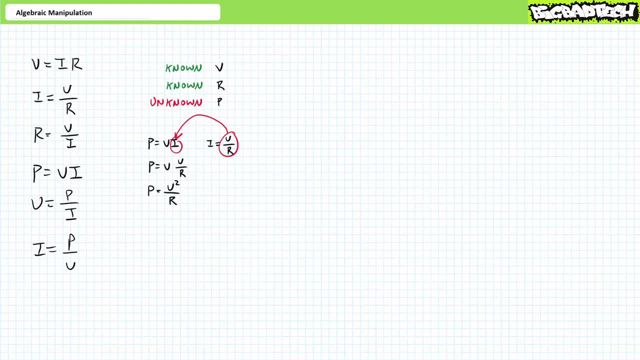 v times v divided by r, which simplifies to p, equals v squared divided by r. Let's say we wanted to solve for unknown p Using the known quantities of i and r. we'll start with one permutation of Ohm's law, which 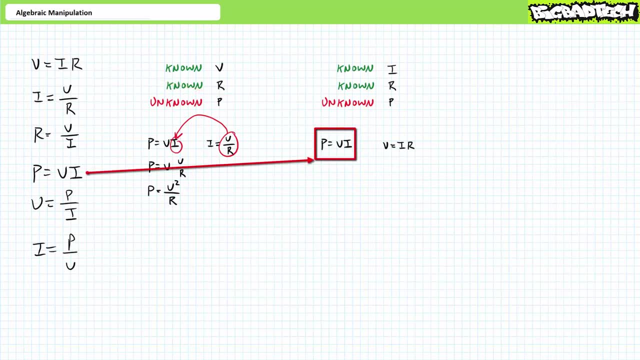 states v equals i times r, and the original DC power equation which states p equals v times i. If v equals i times r, one can substitute i times r in for v into the DC power equation such that p equals i times r times i, which is simplified such that p equals i squared. 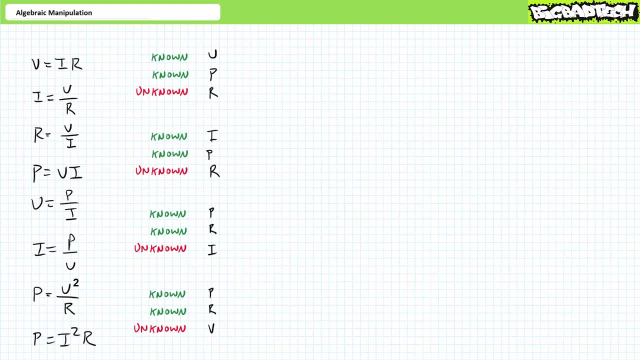 times r. Let's put your understanding of this concept to the test with this series of illustrated example problems. Given, three permutations of Ohm's law, the three original permutations of the DC power equations and these two new permutations- solve for the desired unknown properties in. 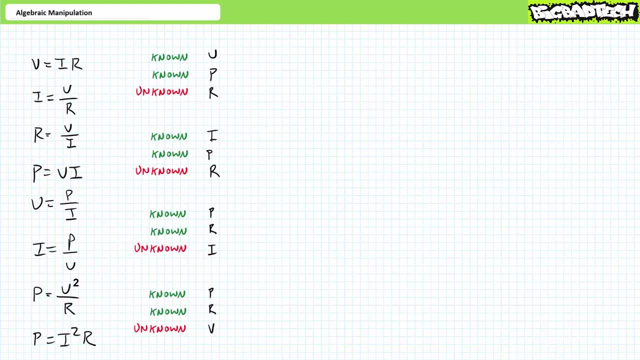 terms of the indicated known properties. The first example is asking us to solve for r in terms of v and p. The second is also asking us to solve for r, but only in terms of i and p. The third problem is asking us to solve for i in terms of p and r. 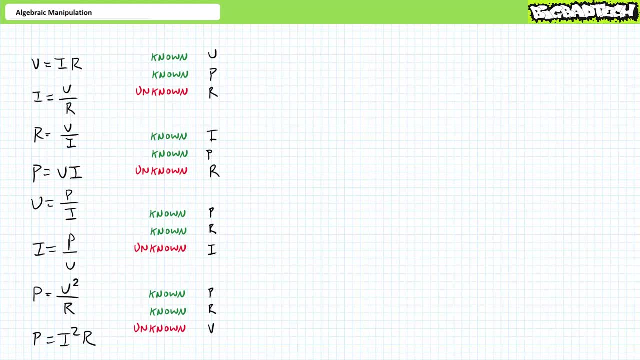 And finally, the last problem is asking us to solve for v in terms of p and r. By all means, pause the lecture and try this on your own. If you're tracking, you should obtain the following results. Our first problem is asking us to solve for unknown quantity r in terms of known p and. 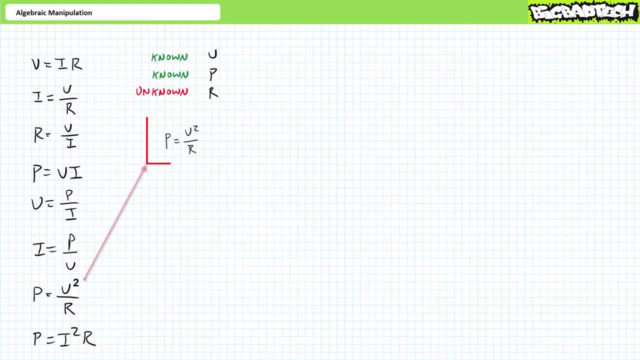 v values. There are multiple places to start. Perhaps the easiest jump off would be one of the newer permutations, where p equals v squared divided by r Solve for r. r is in the denominator. I don't like this. Let's invert both sides. 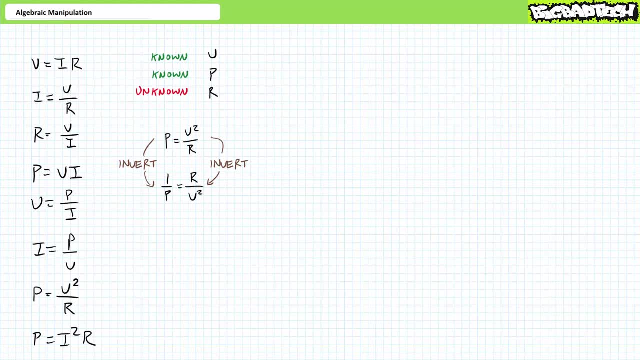 When we flip both sides, we're left with 1 over p equals r divided by v squared. We're left with 1 over p equals r divided by v squared. We're left with 1 over p equals r divided by v squared. 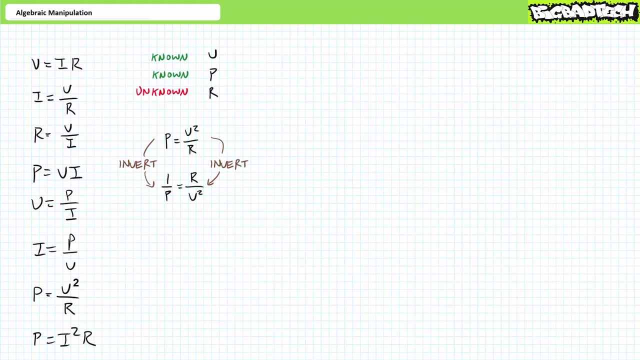 Unknown property r is being divided by v squared. What's the opposite of division: Multiplication. Multiply both sides by v squared. V squared cancels out. on the right, We're left with: r equals v squared divided by p. One can substitute in known values for v and p and determine unknown property r. 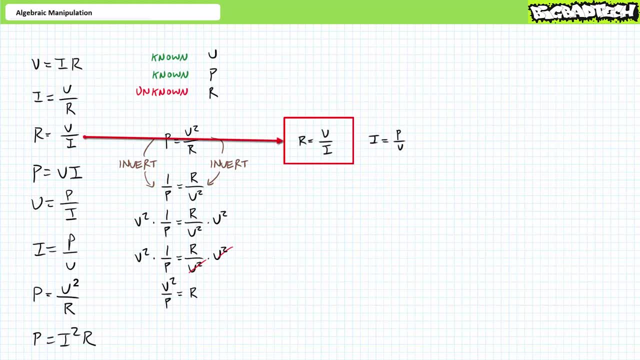 Alternatively, one can begin with one permutation of Ohm's law which states r equals v over i and another permutation of the DC power formula which states i equals p over v. That's all. If i is equal to p over v, one can substitute p over v in for i, which yields a rather ugly. 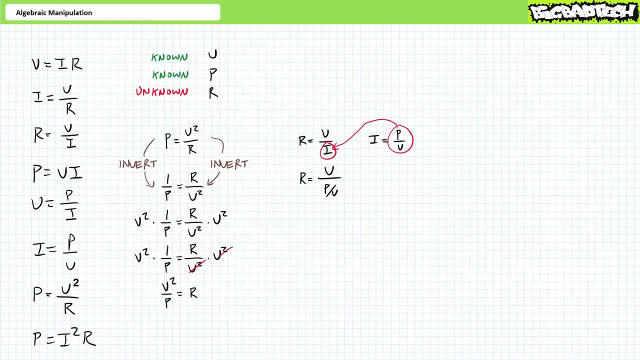 fraction r is equal to v divided by p divided by v. We have got to clean this up. Follow my lead here. Division is the same thing as multiplication by the inverse. This is an extremely handy trick. For example, some quantity to divided by 2 is the same thing as that same quantity times. 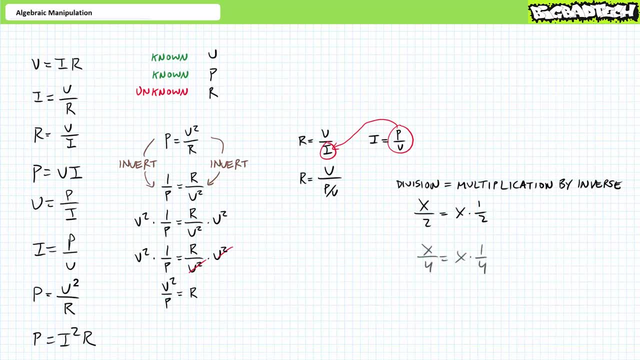 one half, ie the inverse of 2.. Similarly, dividing something by 4 is equivalent to multiplying that same quantity by one quarter. It stands to conjecture: dividing v by p over v is the same thing as multiplying v times the inverse of p over v. 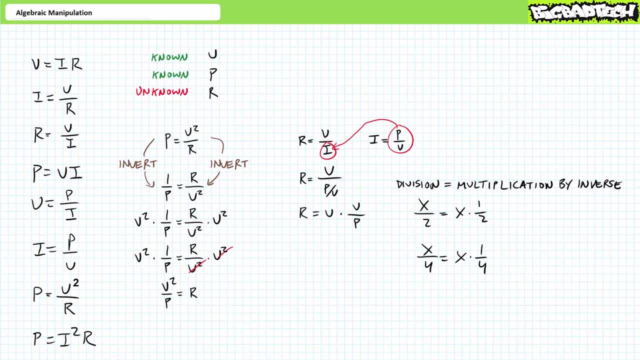 The inverse of p over v is v over p. so we're left with r equals v times v divided by p, which, when simplified, yields r equals v squared divided by p. notably the same result we obtained earlier, albeit by more direct means. 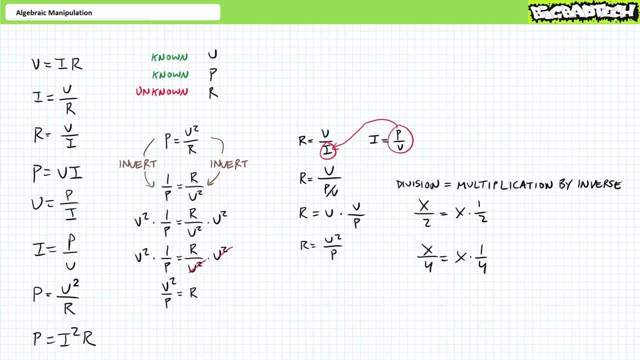 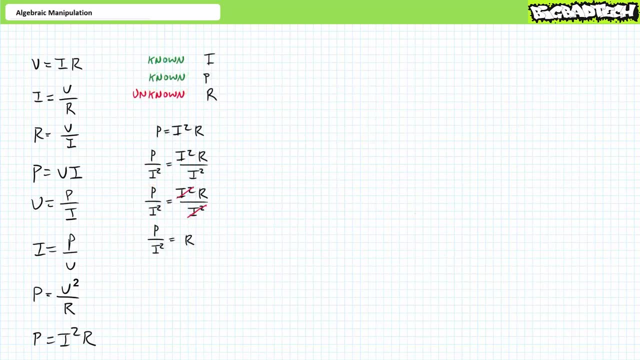 In the interest of time, I'll review the remaining results using the most direct method. Other methods should exist that ultimately yield the same answer, albeit with more or less work. The second problem is asking us to solve for unknown property. r in terms of known properties. 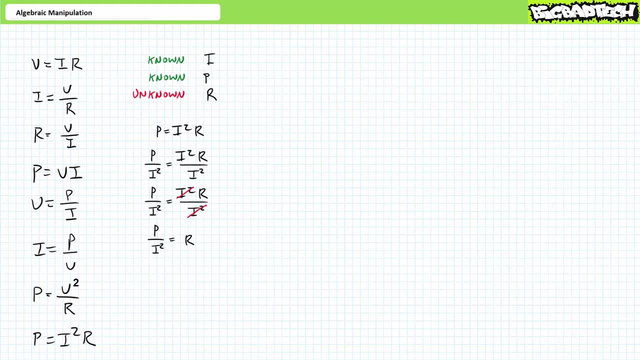 i and p. I started with the equation p equals i squared times. r Divide both sides by i squared. i squared cancels out on the right And we're left with r equals p divided by i squared. The third problem is asking us to solve for unknown quantity. i in terms of known properties. 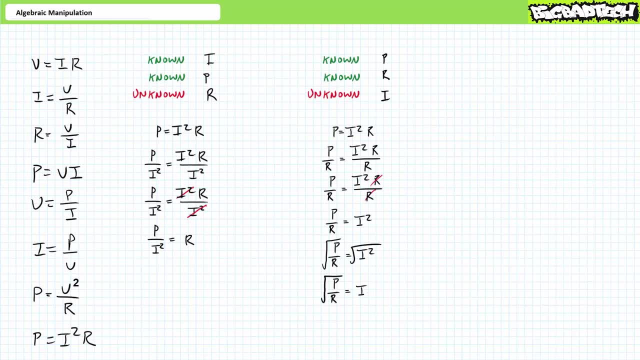 p and r. Again. I started with p equals i squared times r Divide both sides by r. r cancels out on the right and we're left with i squared equals p divided by r. This is not the answer to the problem. 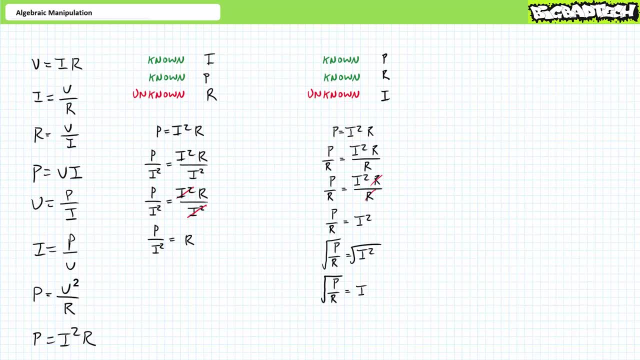 We need to solve for i Take the square root of both sides. Ultimately, we're left with: i equals square root of p divided by r. Note that the terms p over r appear entirely underneath the square root operation. Finally, the last problem is asking us to solve for unknown property: v in terms of known. 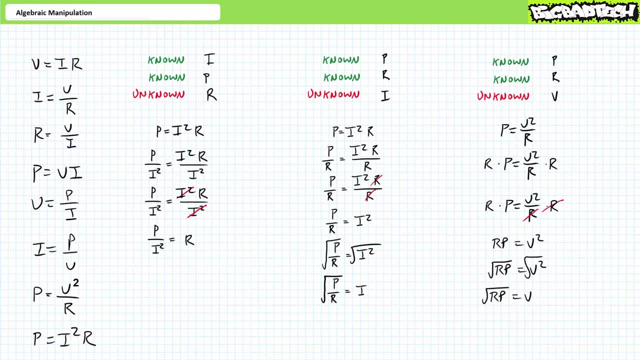 properties p and r. I started with. p equals v squared divided by r. Multiply both sides by r: r cancels out on the right. We're left with v squared equals r times p. Again, this is not the answer to the problem. 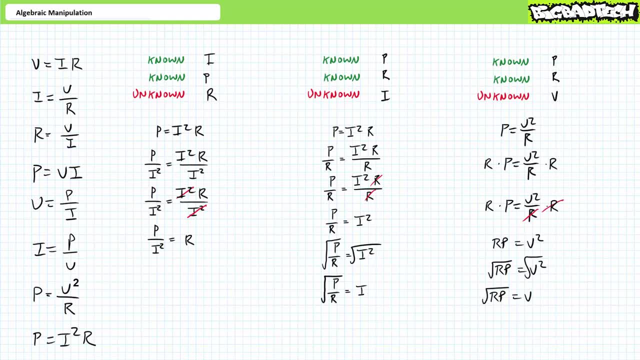 We're looking for unknown quantity v, not v squared Square root both sides. We're left with v equals square root of r times p. Again, note that the term p times r appears entirely underneath the square root operation. For the last problem, we're left with v squared divided by r. 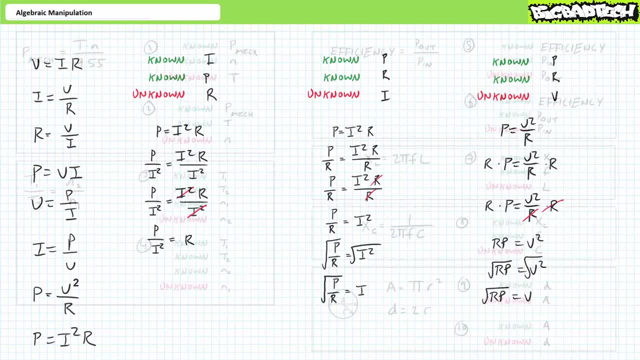 We're left with v equals square root of r times p. We're left with v equals square root of r times p. We're left with v squared divided by r times p. We're left with v squared minus 4.. What does this mean? 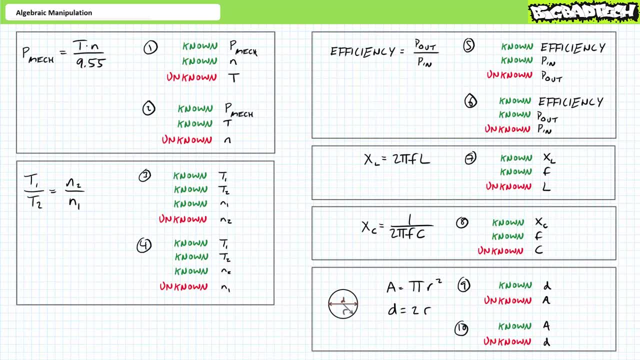 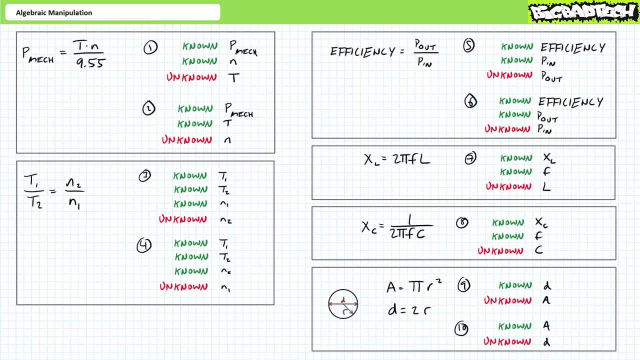 Alright, now that we've got some experience algebraically manipulating similar and slightly more complex expressions, let's try this set of illustrated example problems on for size. Be warned, some of these might be tough. Struggle with them, though. Don't tap out too quick. 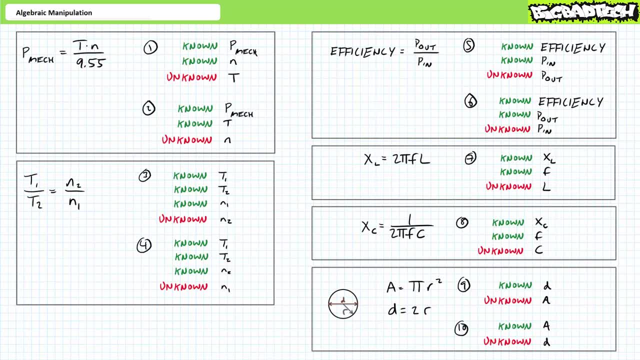 For the purposes of this lecture. don't necessarily concern yourself too much with the concept that these equations represent right now, but rather concentrate today on the process of algebraic manipulation. We'll explore these phenomenon in greater detail in later lectures. Remember, your goal is to isolate the unknowns. 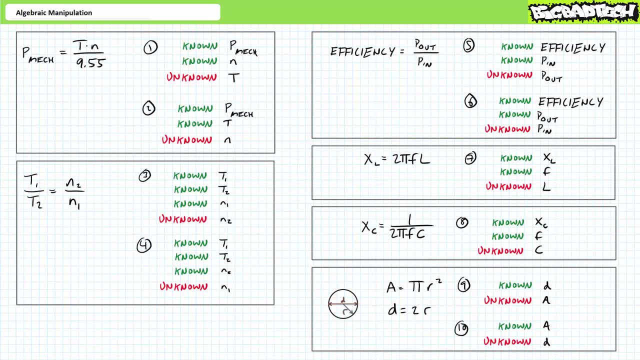 on one side of the equation and the knowns on the other. Quality must be maintained. Don't jam pieces together that don't fit. Any operation you perform on one side of the equation must be performed on the other. Given mechanical power equals T times N divided by 9.55,. 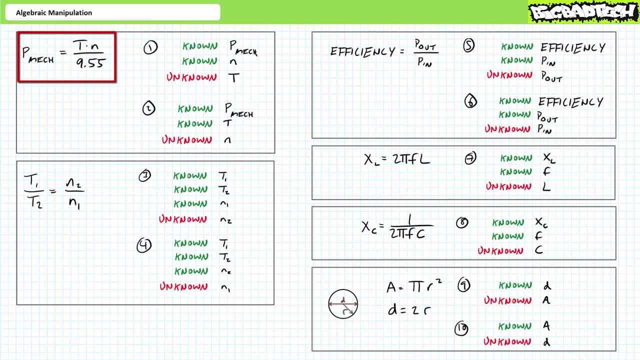 the first problem is asking us to solve for T in terms of mechanical power and N, And the second problem is asking us to solve for N in terms of mechanical power and T. The third problem is asking us to solve for unknown quantity- N2 in terms of known properties. 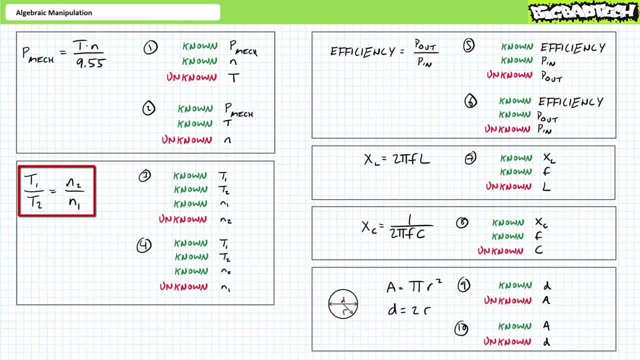 T1,, T2, and N1.. And the fourth problem is asking us to solve for unknown property N1 in terms of known properties N2,, T2, and T1.. Now, don't freak out about these subscripts. T1 is simply a means of differentiating it from T2.. 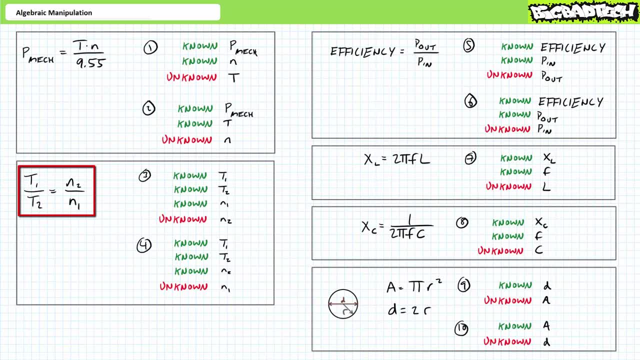 These are not mathematical operators. They're simply subscripts designed to identify certain properties Given. efficiency equals power out over power in. the fifth problem is asking us to solve for unknown property: P out in terms of known properties, P in and efficiency. And the sixth problem is asking us to solve for unknown property: 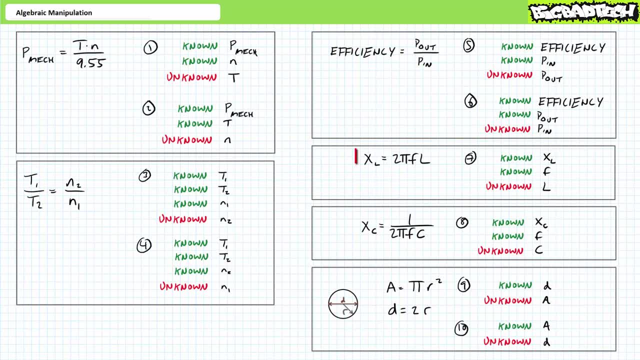 P in in terms of known properties, P out and efficiency. Given x sub l equals 2 pi times f times l. the seventh problem is asking us to solve for unknown property l in terms of known properties f and x sub l. given X sub C equals one divided by two pi F times C. 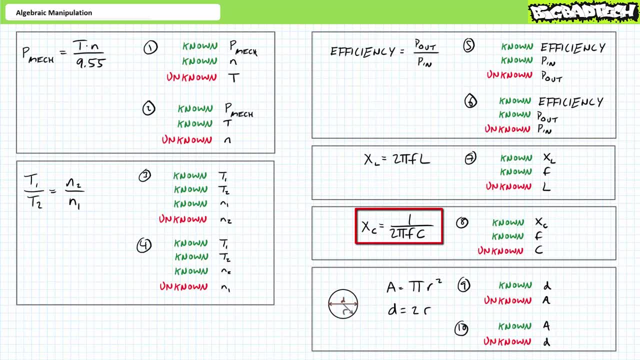 Problem eight is asking us to solve for unknown property C, given known properties F and X sub C. Lastly, given a circle with area of pi times R squared and the fact that diameter is two times the radius, problem nine is asking us to solve for area. 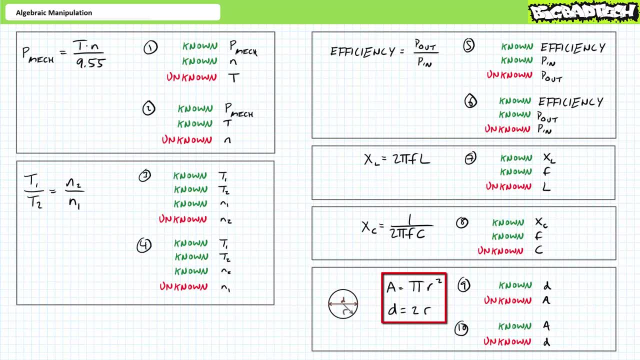 in terms of diameter, And problem 10 is asking the reverse solve for diameter in terms of area. By all means, pause the lecture and try this on your own. If you're tracking, you should obtain the following results. Our first problem features: 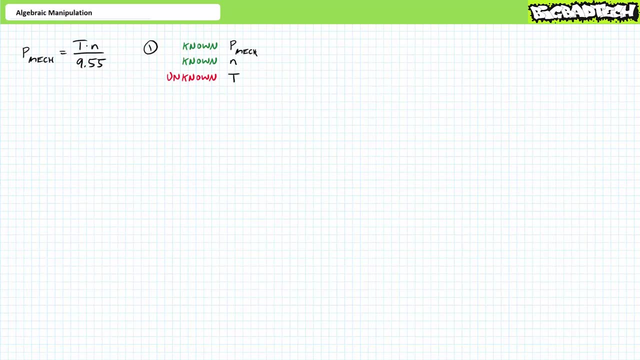 the rotating mechanical power formula which states: rotating mechanical power is equal to torque T times rotational speed, N divided by 9.55.. We're being asked to solve for unknown torque, given known mechanical power and known speed, Unknown property, T is being multiplied by N. 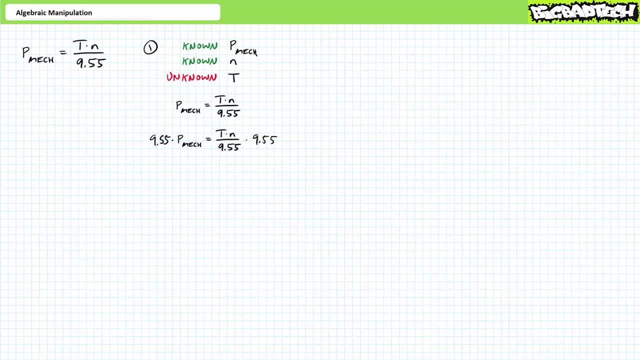 and divided by 9.55.. Multiply both sides by 9.55.. 9.55 cancels out on the right. divide both sides by N. N cancels out on the right and we're left with T equals 9.55. 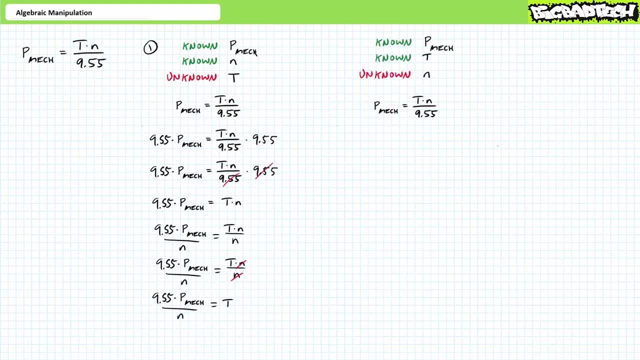 times mechanical power divided by N. Our second problem is asking us to solve for unknown property, N, given known T and mechanical power values. Multiply both sides by 9.55.. 9.55 cancels out on the right. Divide both sides by T. 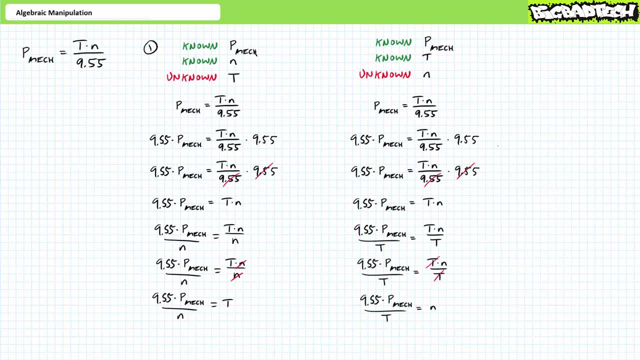 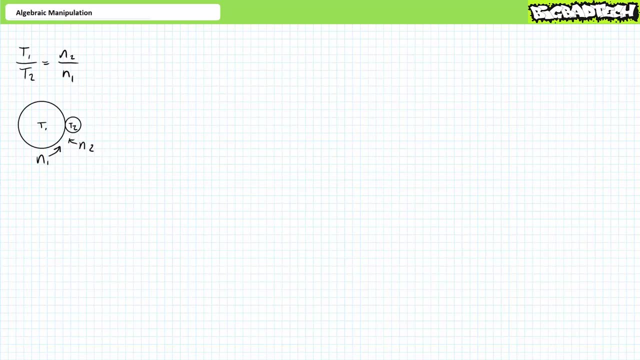 T cancels out on the right and we're left with N equals 9.55 times mechanical power divided by T. Our second problem involves gear ratios, where the number of teeth on gear one divided by the number of teeth on gear two is equal to the rotational speed of gear two. 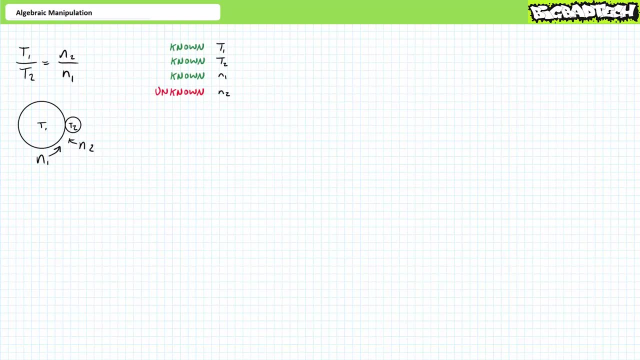 divided by the rotational speed of gear one We're being asked to solve for unknown property N2, given known properties N1,, T2, and T1.. Given T1 over T2 equals N2 over N1,. multiply both sides by N1,. 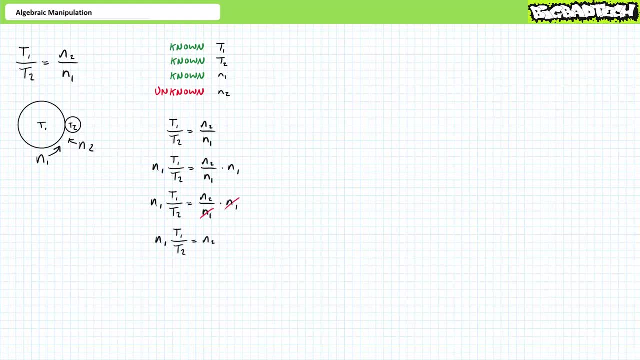 where N1 cancels out on the right, where we're left with unknown property N2 equal to N1 times T1 over T2.. Our next problem is asking us to solve for unknown property N1, given known properties N2, T2, and T1. 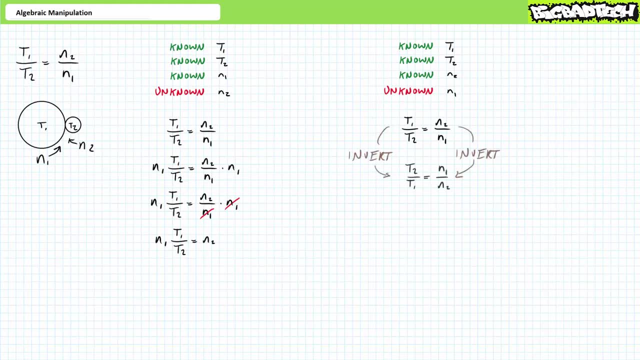 Again, given T1 over T2 equals N2 over N1, one may initiate this algebraic manipulation by inverting both sides. Multiply both sides by N2, N2 cancels out on the right, and we're left with N1 equals N2 times T2 divided by T1. 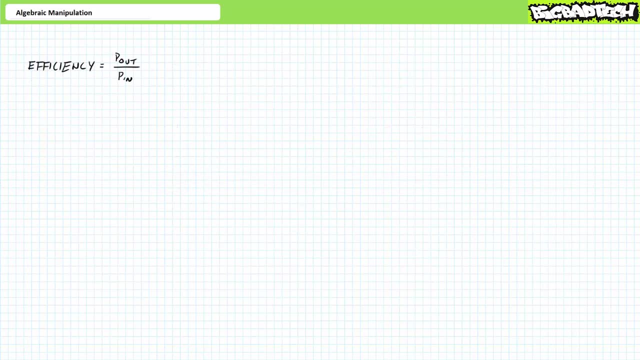 Our next problem is asking us to solve for unknown property N1, given known properties N1,, T2, and T2.. The next problem deals with the ratio of efficiency, or efficiency is equal to the power out- P out- divided by the power in- P in. 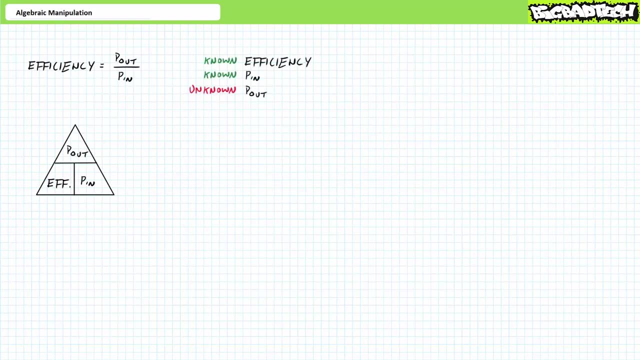 It's perhaps easiest to set this up in a triangle format. We're first being asked to solve for unknown property, P out. given known properties, P in and an efficiency Solve for P out by covering up P out. P out is equal to P in times: efficiency. 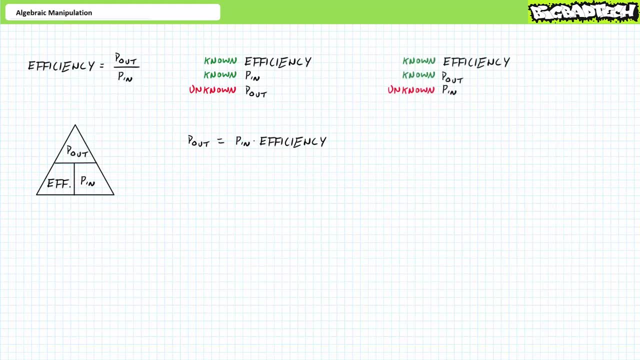 because efficiency is side by side with P in. The next problem asks us to solve for P in. given known properties. P out and efficiency cover up P in. P in is equal to P out over efficiency because P out is over efficiency. 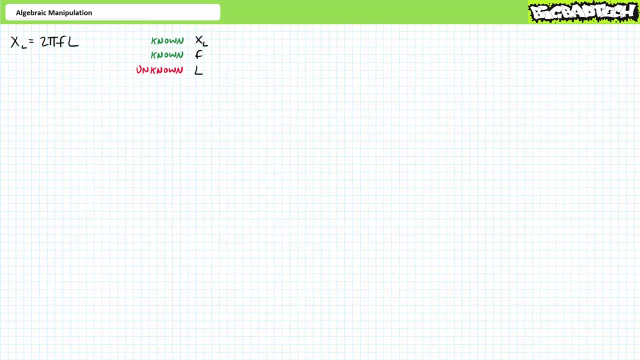 Our next problem demonstrates that X sub L is equal to two pi times F times L. We're being asked to solve for unknown property L in terms of the known properties F and X sub L. Again, don't freak out by the subscript. L is not a mathematical operator. 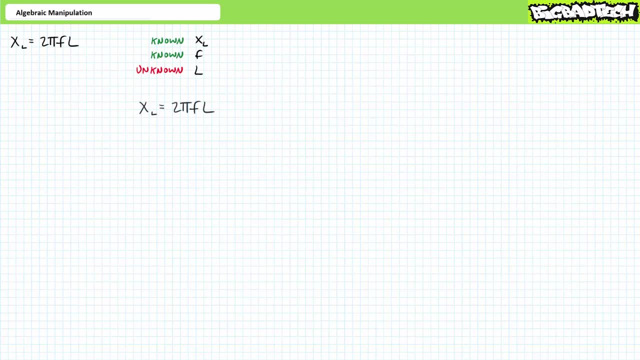 It's simply a means of identifying property X. X sub L equals two pi times F times L. Unown property L is being multiplied by two pi F, Divided both sides by two pi F. You can do this all at once or one at a time. 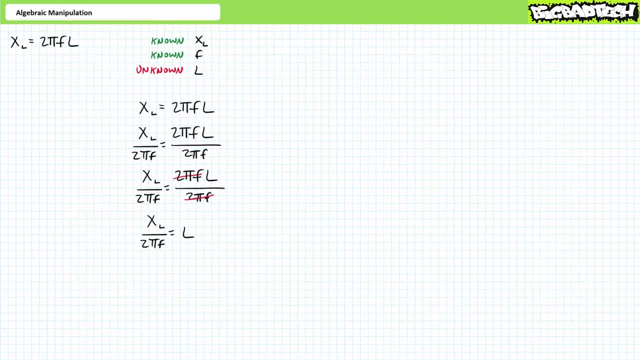 Two pi F cancels out on the right-hand side And we're left with L equals X sub L divided by two pi F. Given X sub C is equal to one divided by two pi F C. we're being asked to solve for unknown property, C. 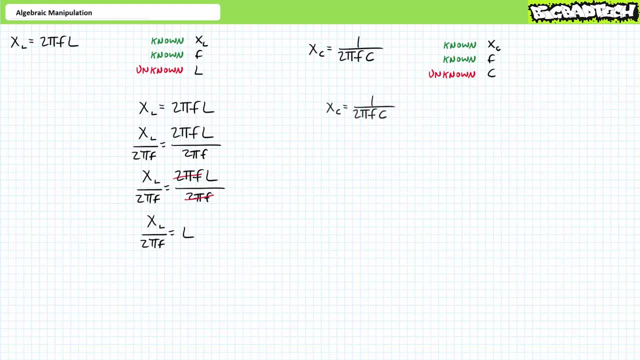 in terms of known properties F and X sub C. Given X sub C equals 1 over 2 pi f c, perhaps the easiest way to start is to invert both sides such that 1 over x sub c equals 2 pi f c. 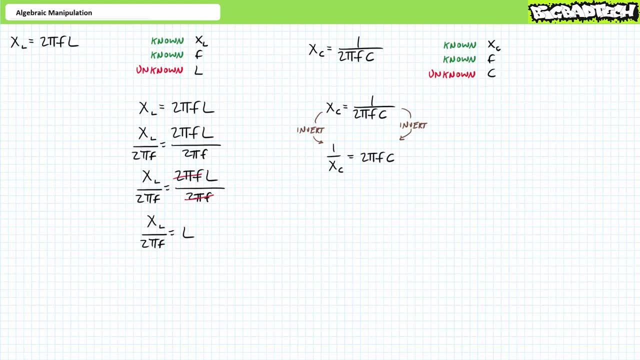 Unknown property, c is being multiplied by 2 pi f. Dividing both sides by 2 pi f, we're left with a rather ugly fraction: 1 over x sub c, divided by 2 pi f on the left-hand side. It's important to remember division is equal. 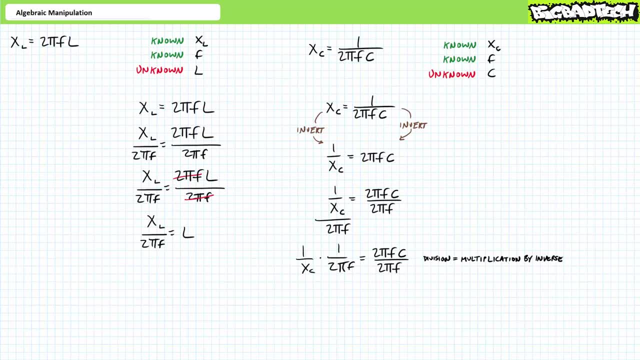 to multiplication times the inverse. What's the inverse of 2 pi f? The inverse is 1 over 2 pi f. So 1 over x sub c divided by 2 pi f is equivalent to 1 over x sub c times 1 divided by 2 pi f. 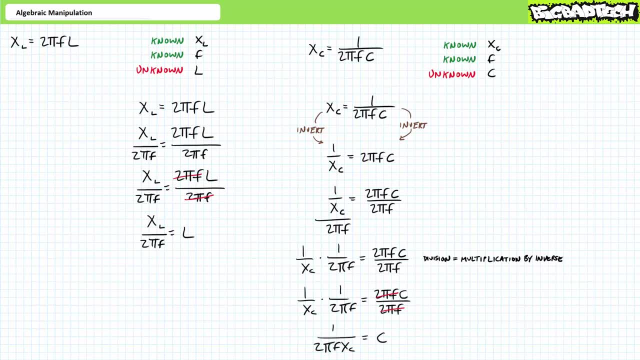 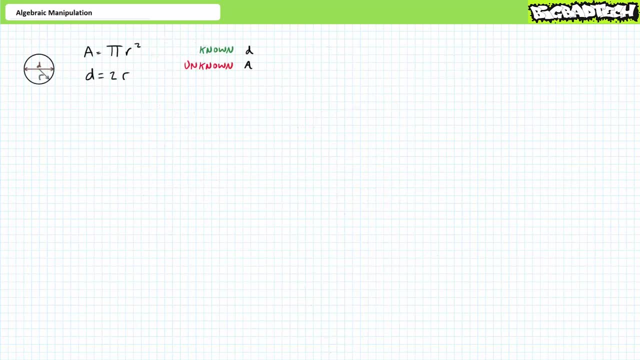 2 pi f cancels out on the far right-hand side, such that unknown property c is equal to 1 over 2 pi f times x sub c. Our next problem demonstrates the area of a circle is equal to pi times the radius squared. 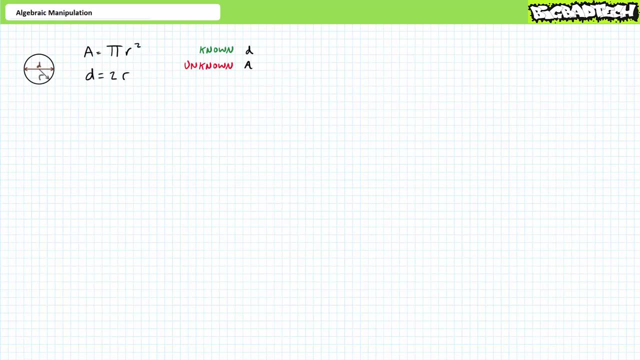 Additionally, we're aware that its diameter is equal to 2 times the radius. We're being asked to solve for unknown property a in terms of known property d. With very little effort it could be demonstrated: radius is half of diameter, so r equals d divided by 2.. 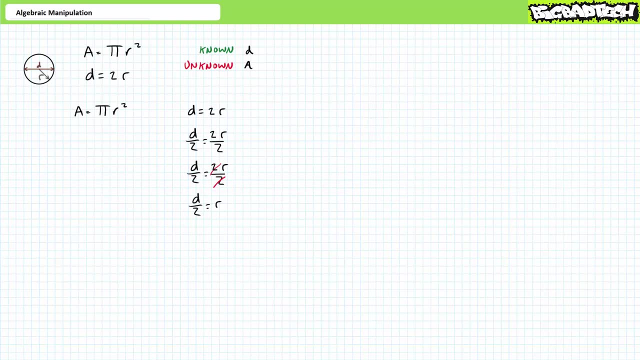 Now, given our area expression, where area of a circle is equal to pi times radius squared, we can substitute d over 2 in for r, which yields area equals pi times d divided by 2 squared. Note the parentheses: D divided by 2 times d divided by 2 is d squared divided by 4,. 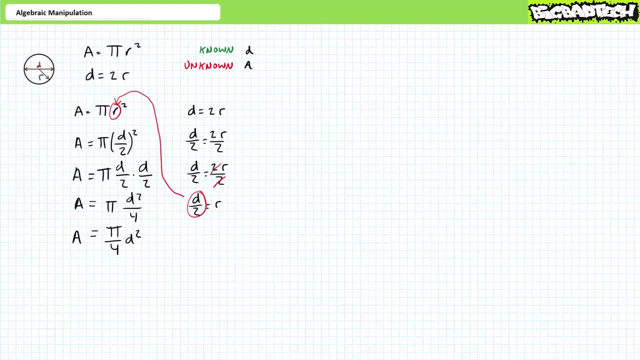 which some mathematical purists will rearrange, since the constants appear together such that area equals pi over 4 times d squared. Lastly, we're being asked to solve for unknown property, d given, known property, a, Given. we previously demonstrated that a equals pi. 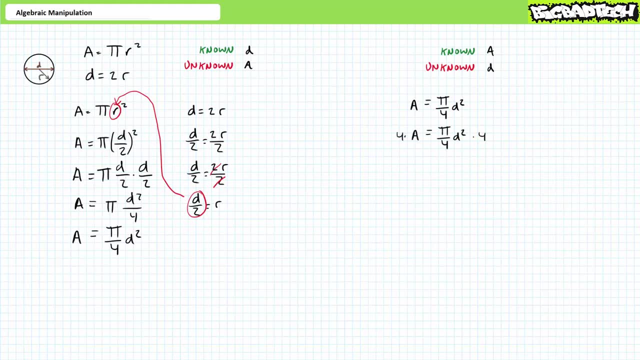 over 4 times d squared. multiply both sides by 4.. 4 cancels out on the right. Divide both sides by pi. Pi cancels out on the right, leaving us d squared equals 4 times area divided by pi. This is not the answer we're looking for. 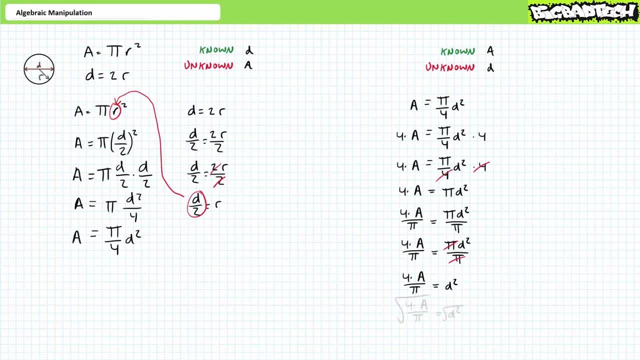 This is the software for d squared. We need to solve for property d. Take the square root of both sides, which yields d equals square root 4 times area divided by pi, which some mathematical purists may take the square root of 4 and write this as 2 times the square root. 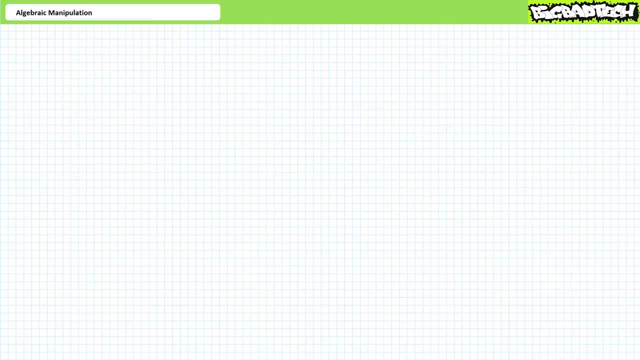 of area divided by pi. All right, that might have been a little tough for some of you. Again, keep in mind this general guidance about algebraic manipulation: Isolate unknowns on one side of the equation and all the knowns on the other. 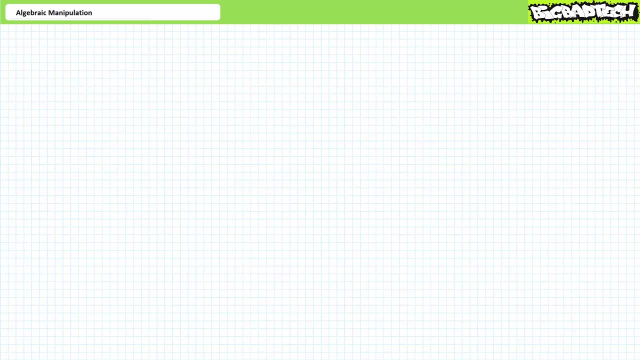 Follow the rules. when doing so, Equality must be maintained at all times. Any operation performed on one side must also be performed on the other. Lastly, don't forget what you're solving for. Too often, I've observed individuals struggling with this topic. perform some operation one step only. 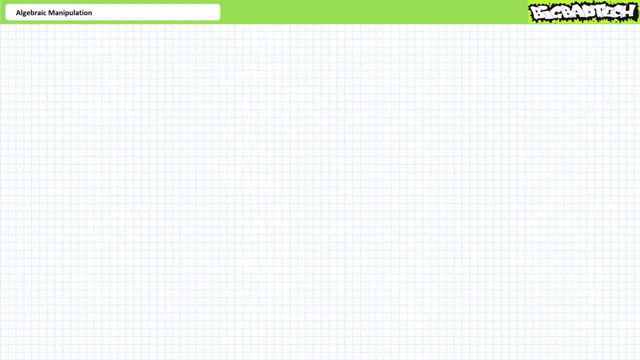 to undo it. By annotating each step of the manipulation process, you can backtrack and correct any mistakes you may have made. Before we bring this lecture to a close, let me answer a burning question that might have been in the back of your mind since you first learned algebraic manipulation. 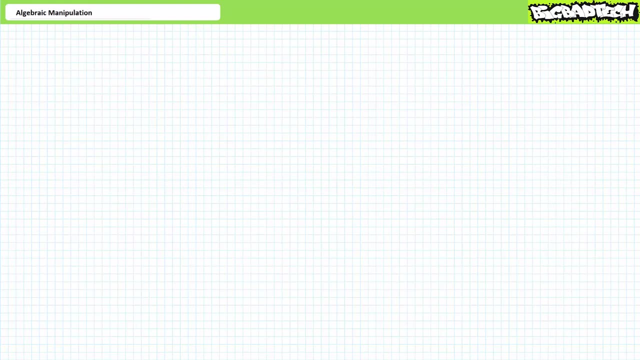 way back in grade school, That question being: why are we doing this? This deserves an answer, because the larger purpose may not be readily apparent so early in this lecture series. Your math teacher's goal in high school really was to frustrate and humiliate you. 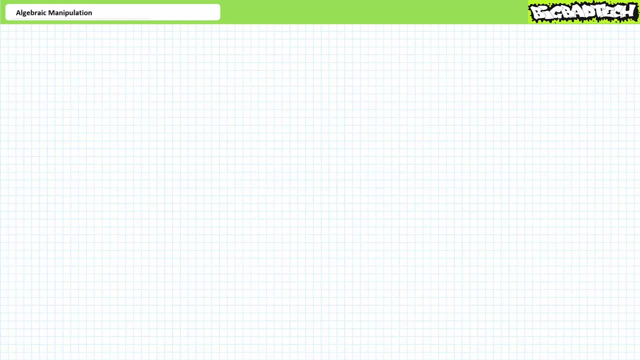 My purpose in reviewing this lecture is to help you understand why you're doing. algebraic manipulation is because it's used on a very frequent basis. Given an accepted relationship between certain properties and known values, one can solve for unknown properties. A simple example: 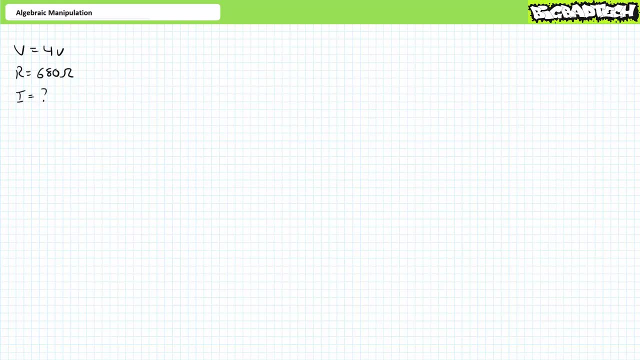 Calculations can take the place of equipment Given: 4 volts across a 680 ohm resistor, what's the current through it Given? Ohm's law demonstrates that I equals V over R. 4 volts divided by 680 ohms yields roughly 5.9 milliampers. 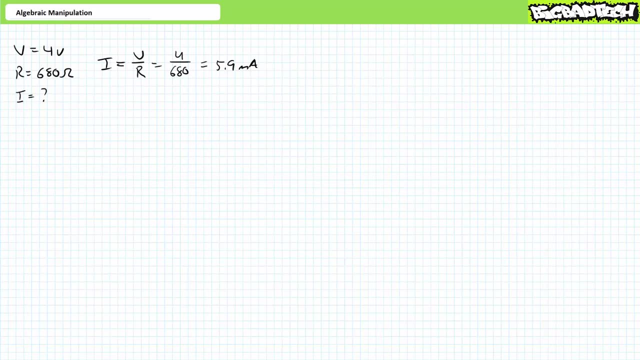 If you know voltage and resistance, you don't have to use an ammeter to measure current. You can calculate it. A slightly more complicated example: Will the part work? Oftentimes rated mechanical power and rated speed appear on a motor nameplate, but rated torque is unlisted. 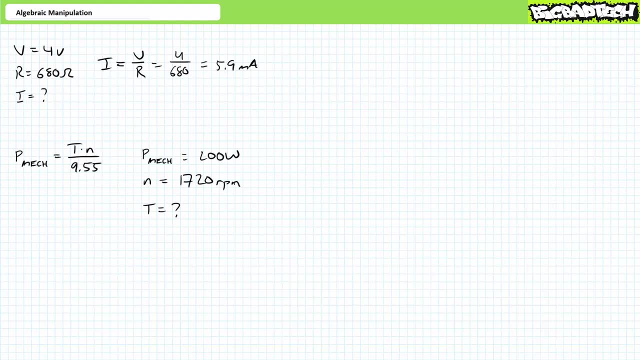 Does a 200 watt motor operating at 1720 RPM have enough torque to do the job Given? mechanical power is equal to torque times rotational speed divided by 9.55.. We demonstrated via algebraic manipulation that torque equals mechanical power times 9.55 divided. 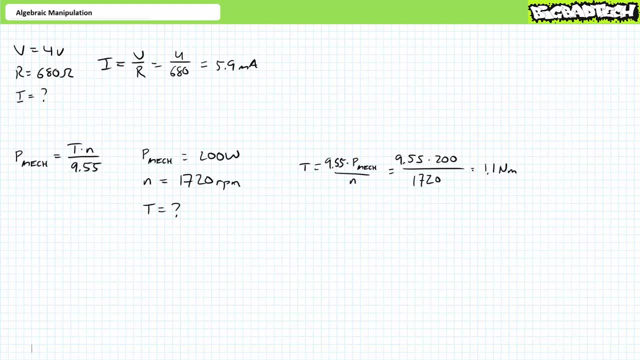 by rotational speed Substituting 200 watts and 1720 RPM demonstrates this motor is capable of producing roughly 1.1 newton meters of torque at the rated condition. Does the job require 1.1 newton meters of torque or less? 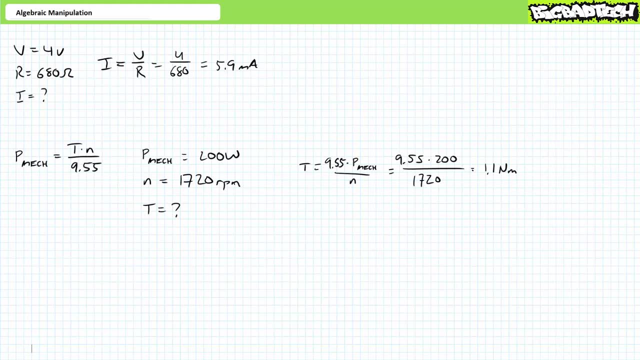 It should be good. Does the job require more than 1.1 newton meters of torque? Go get a bigger motor. Here's yet another example. What part do I need? Let's say we need to find a motor that has a torque of 1.1 newton meters. 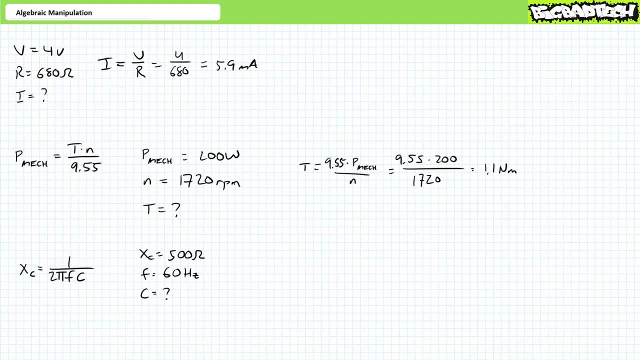 Let's say we need to find a motor that has a torque of 1.1 newton meters. Let's say we need to find which capacitance value will provide 500 ohms of impedance at 60 hertz frequency. The capacitive impedance magnitude equals 1. 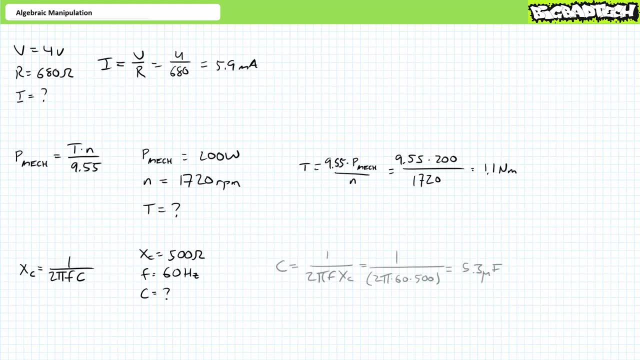 over 2 pi times the frequency times the capacitance value. We demonstrated via algebraic manipulation that C equals 1 over 2 pi times F times X sub C. Substituting in the known values for X sub C in frequency demonstrates that roughly 5.3 microfarad capacitor should do the trick. 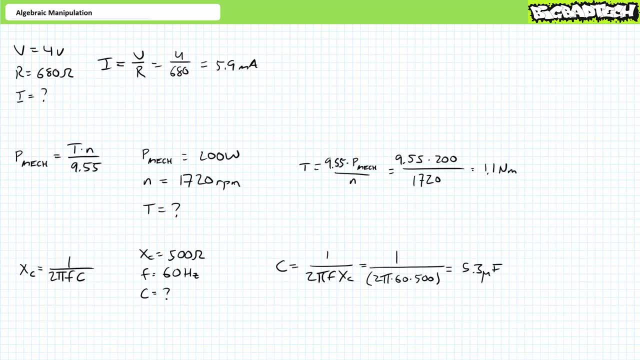 We'll examine many practical applications like this and more as we progress forward. In conclusion, this lecture presented a review of algebraic manipulation. We learned algebraic manipulation is the process of rearranging an expression such that all unknown properties are on one side of an equal sign.